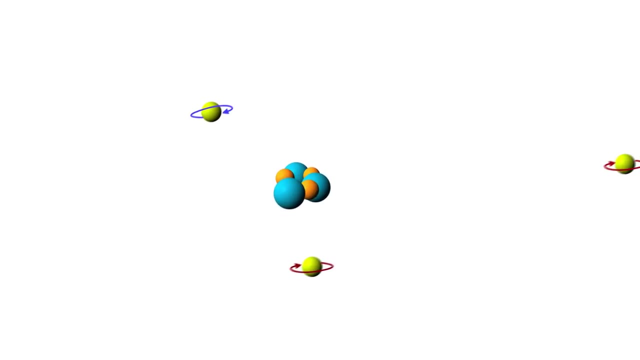 as it does. spinning counterclockwise, their magnetic fields cancel each other out, So an atom needs an imbalance of electrons spinning in different directions to generate a magnetic force. The larger the difference in spinning electrons in a random atom, the stronger the magnetic force. The magnetic force forms a field around the atom. 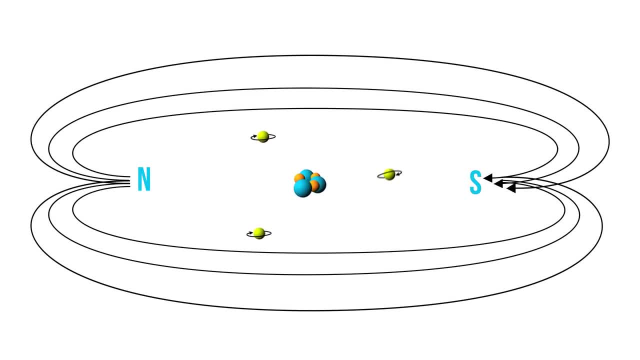 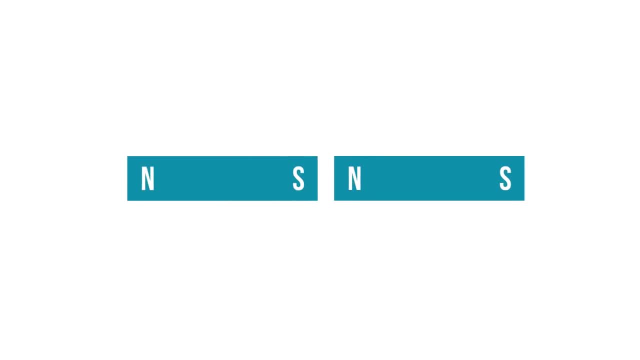 The field begins at the north pole and is terminated at the south pole, continuing through the magnet. When two magnetic atoms are near each other, they interact. Their like poles repel or their unlike poles attract. As atoms attract, they align and their magnetic fields add together, creating a stronger magnetic force. 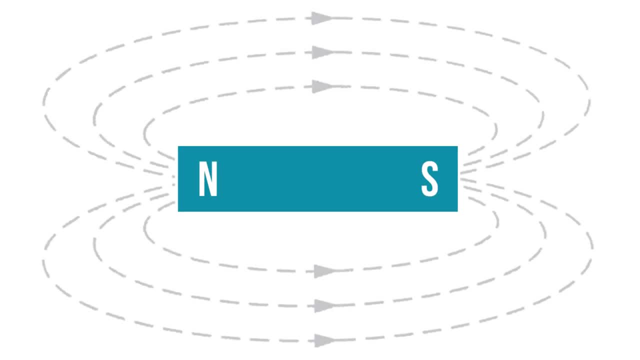 The magnetic field is made up of lines of force collectively referred to as magnetic flux. The flux lines are not physical but demonstrate the strength of the magnet or magnetic field. Here I've poured iron filings onto a piece of paper on top of a bar magnet. 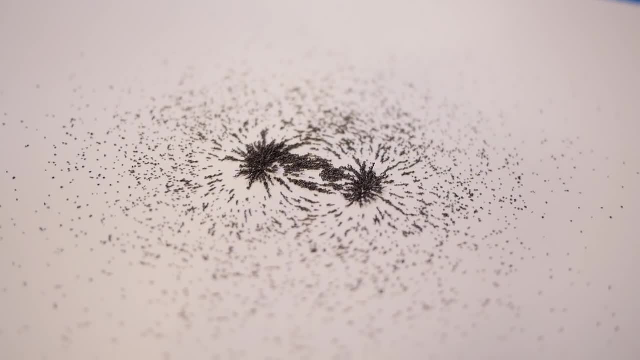 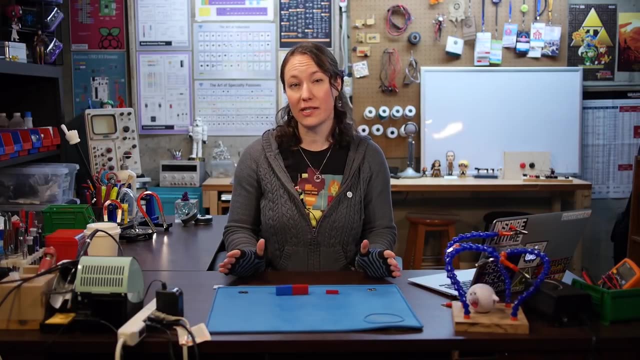 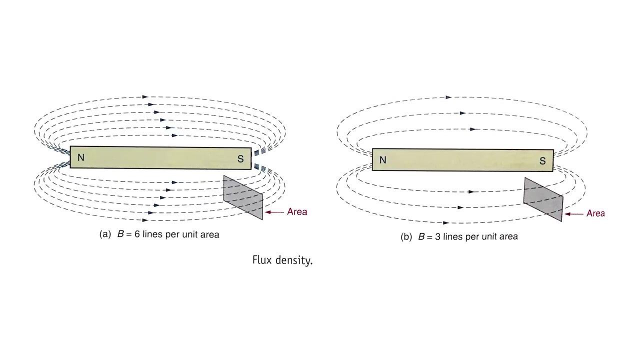 The iron is attracted to the magnetic field. Can you see the lines? The strength of a magnet's force is determined by the size of its magnetic field and the amount of flux that field contains, also known as flux density. The greater the number of flux lines per unit of cross-sectional area, the stronger the 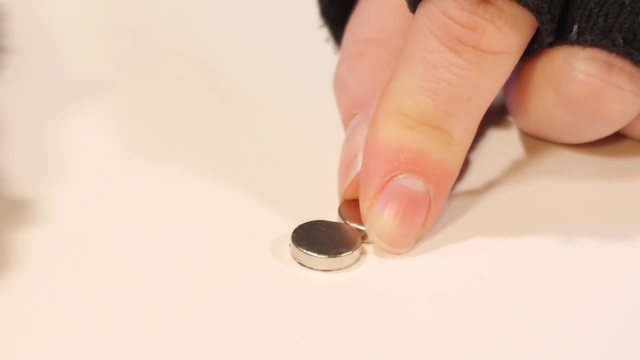 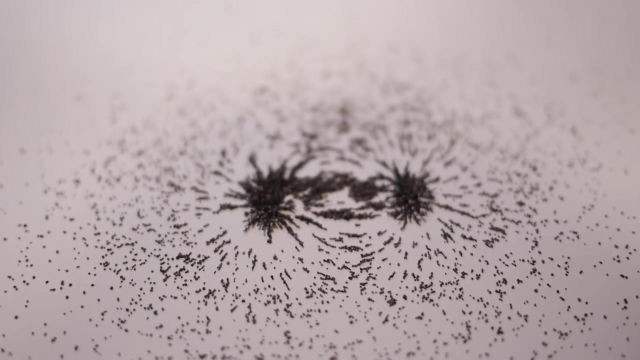 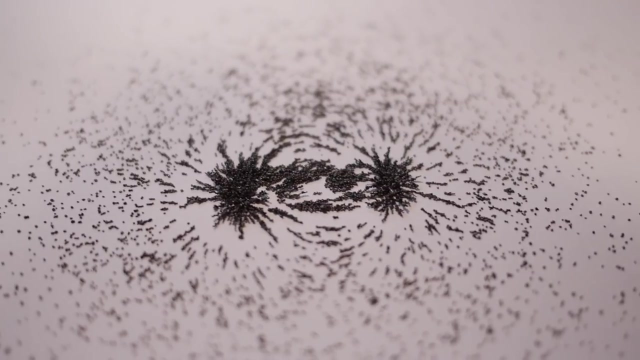 magnetic force. Neodymium magnets are harder to pull apart than ceramic magnets. They are stronger and therefore have a higher flux density. Flux density is greatest at a magnet's poles than anywhere else in its magnetic field. You can see how more iron filings are drawn to the poles of the magnet. 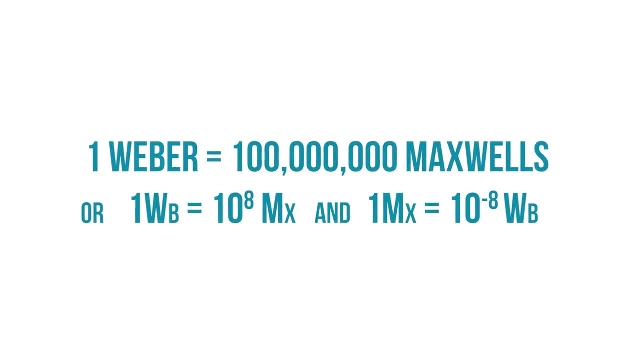 Scientists and engineers express the overall magnitude or quark of a magnet. They may use the measurements of the actual magnetic force and the quantity of a magnetic field in units of Weber's for strong fields or Maxwell's for weak fields. 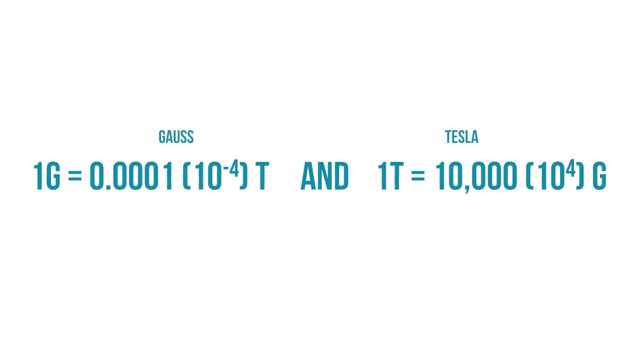 But more often flux density is measured in Teslas or Gauss. These units define the concentration or intensity of the magnetic field. A Tesla is defined as one Weber of flex per square meter. In equations, flux density is represented by a capital B. Some materials respond to the presence of a magnetic force, while others are not. Here's an example by a magnet. where we have an iron, The magnet must be an iron or iron as it moves forward and forwards. If the iron is not an iron, the magnet must be a magnet. 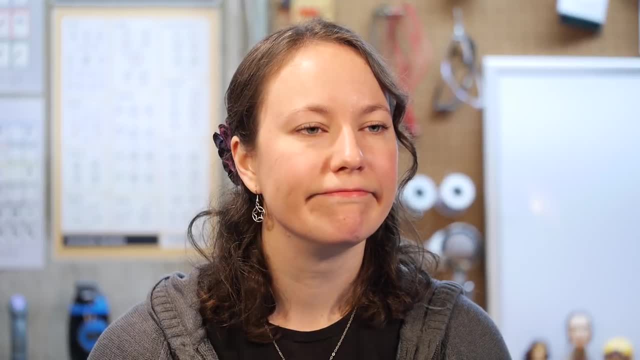 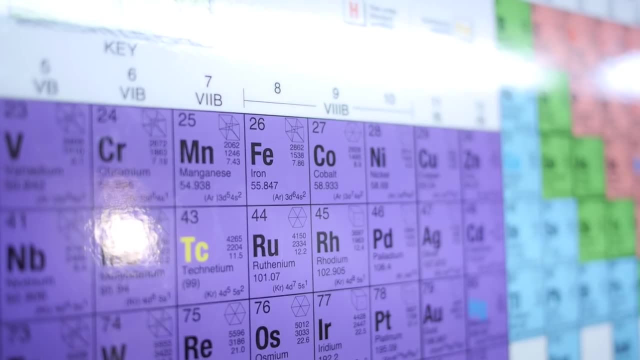 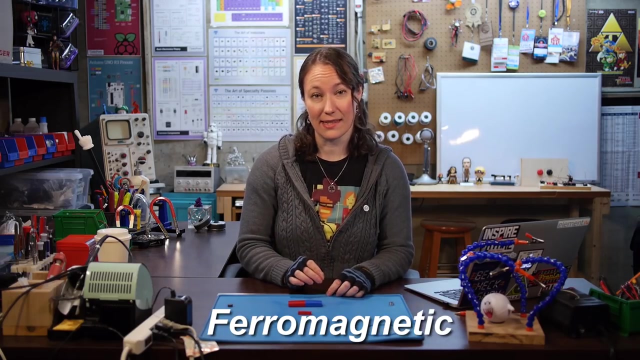 do not. You may have heard of ferrous metals, Bueller, Bueller, Not that kind of ferrous Ferrous as in Fe. Ferrous metals are those that contain iron. Iron is a ferromagnetic substance, meaning it has an extremely high relative permeability. 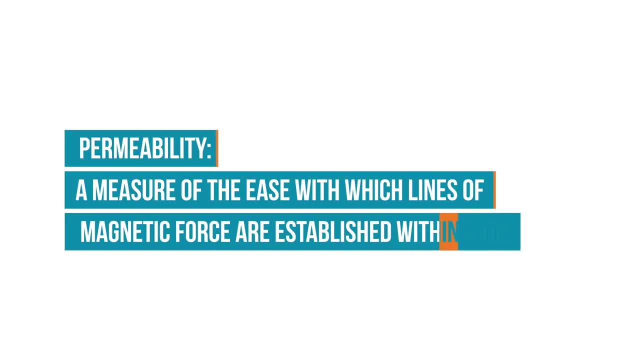 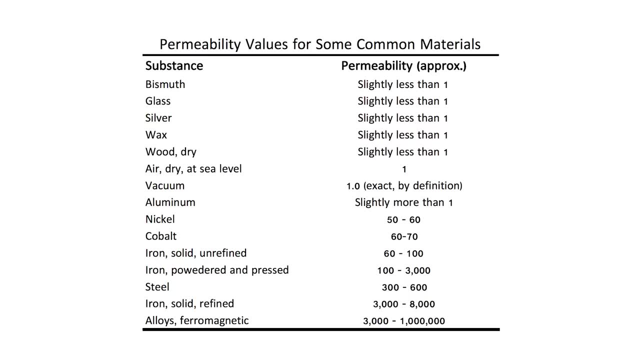 rating Permeability is a measure of the ease with which lines of magnetic force are established within a material. A material's permeability is usually measured relative to the permeability of free space, A substance that causes flux lines to bunch together more tightly than free space would be. 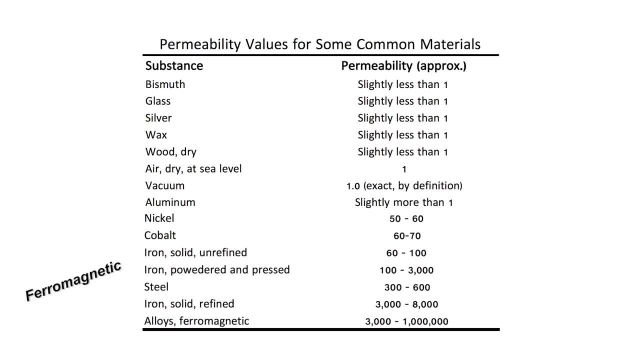 ferromagnetic. Ferromagnetic materials include iron, cobalt and nickel. Free space has a rating of 1.. Materials with relative permeability ratings slightly greater than 1 are considered paramagnetic. Paramagnetic materials include gold, aluminum and copper. Materials with relative permeability. 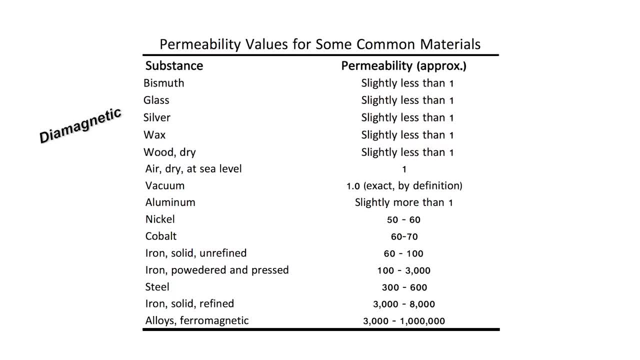 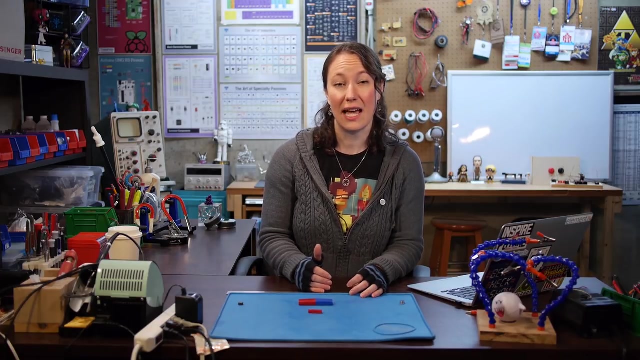 ratings that are less than 1 are called diamagnetic. These include anything that does not react to the permeability of free space. However, no diamagnetic material exists that can decrease the strength of a magnetic field as much as a ferromagnetic material can increase it. This will be important to 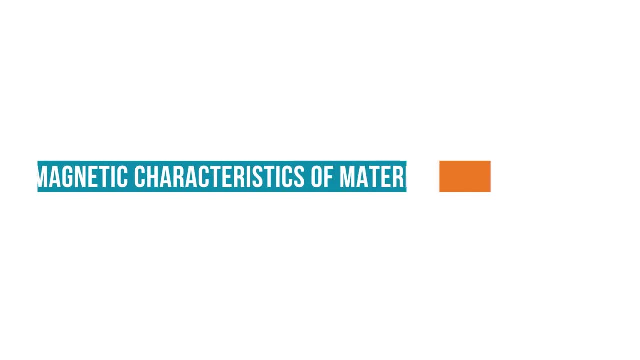 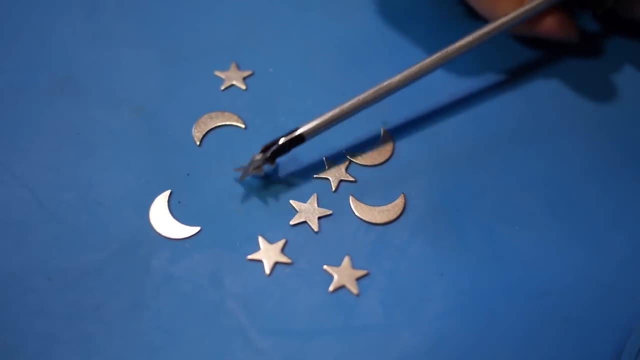 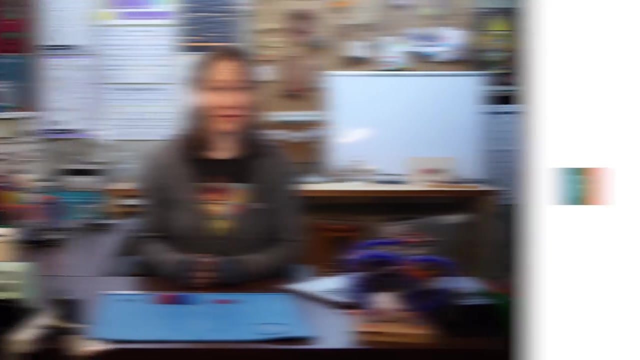 consider later when we talk about magnetic shielding. Have you ever rubbed a magnet on a piece of metal and found out that afterwards other pieces of metal would stick to it? This is because it's possible to magnetize an object simply by placing it within the field of a magnet. Reluctance is the resistance of a material to magnetic. 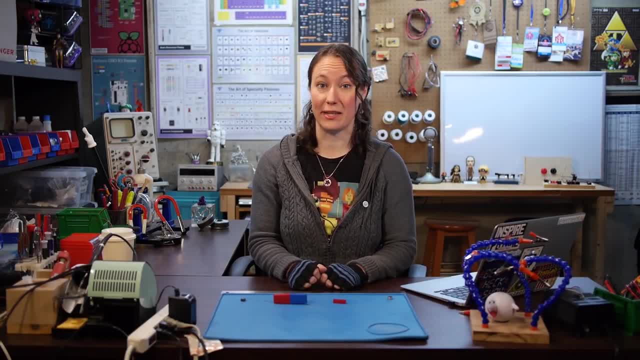 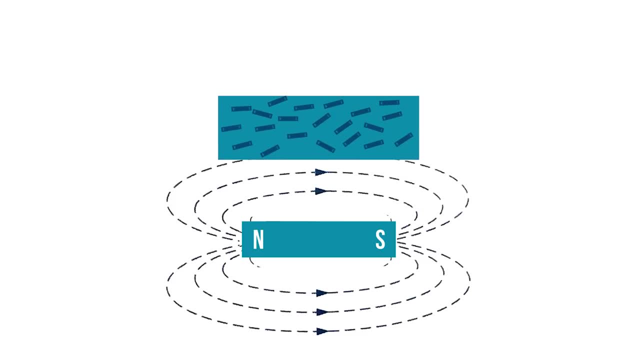 lines of force. Materials with a low reluctance can be easily magnetized. When a low-reluctance material is placed in a magnetic field, the poles of the magnet act upon the atoms within the material. The unlike poles between the atoms and the magnet attract. 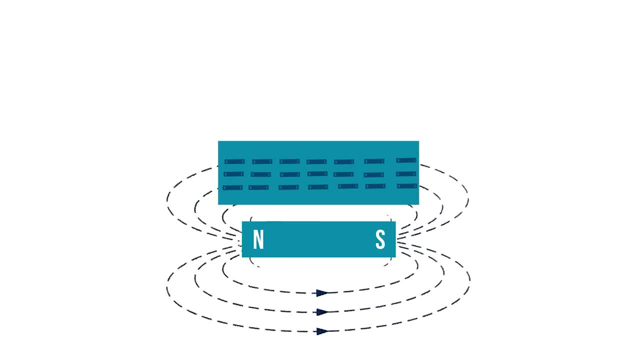 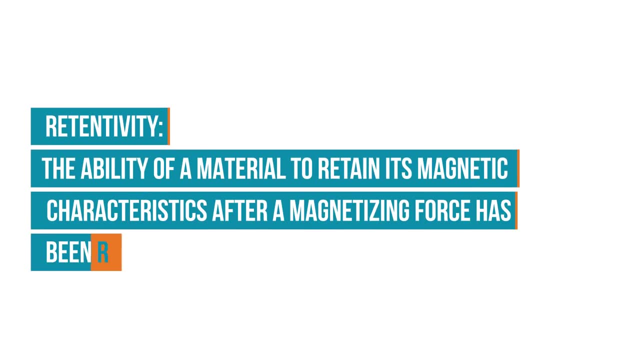 like in a magnet, the atoms align, increasing the magnetic field of that material, and the material becomes temporarily magnetized. The material's retentivity determines how well it stays magnetized once the magnet has been removed. High-permeability materials have a low 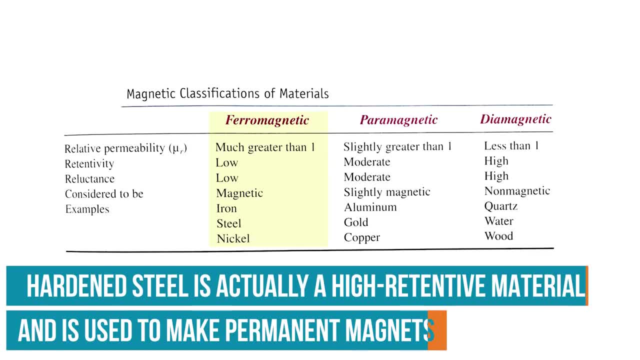 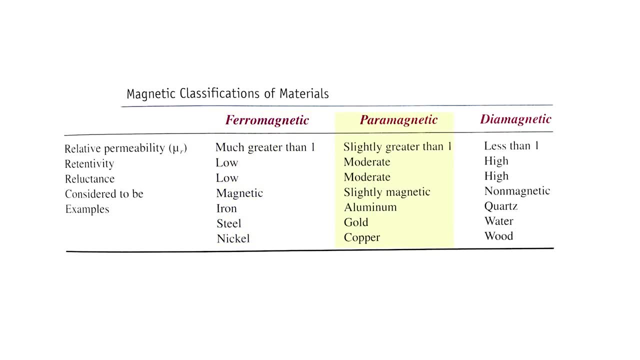 reluctance and are therefore easily magnetized. But they have a low retentivity, so they quickly lose their magnetic strength. Low-permeability materials have a high reluctance and are therefore difficult to magnetize. However, they do have a high retentivity, which means that the 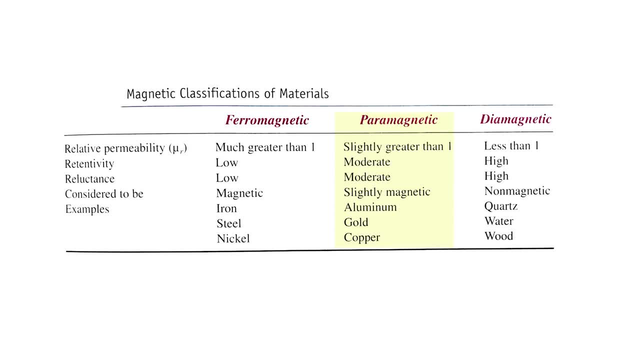 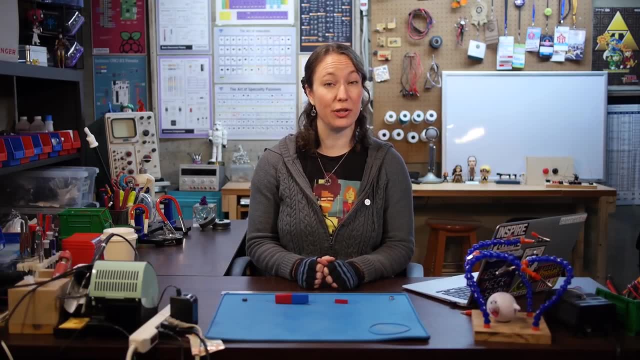 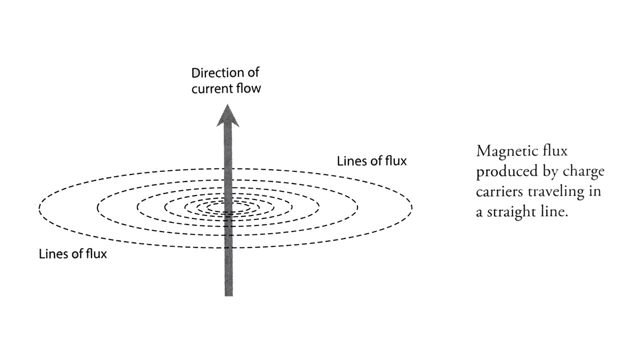 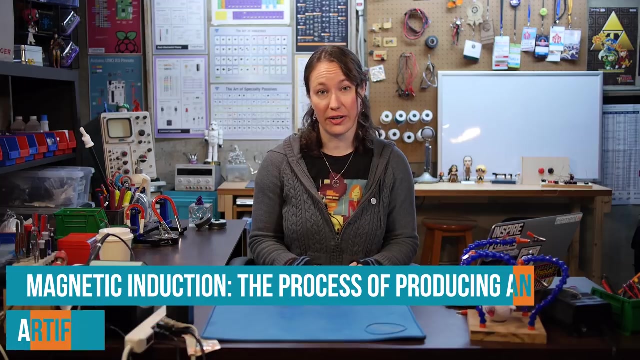 magnets retain their magnetic strength for a long period of time. Most magnets are artificially produced by some external source. Since electrons have magnetic fields, their motion, like an electric current flowing through a wire, also produces a magnetic field or flux. One way to create a magnet is by using a strong DC current. 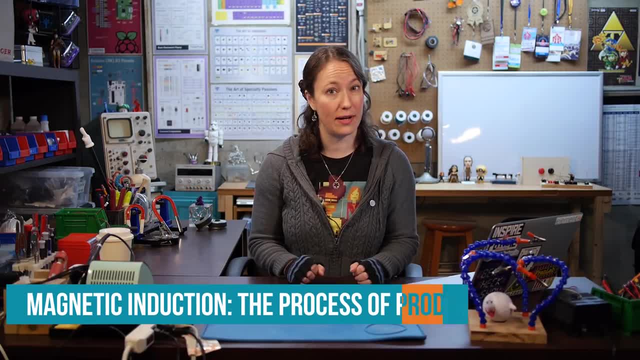 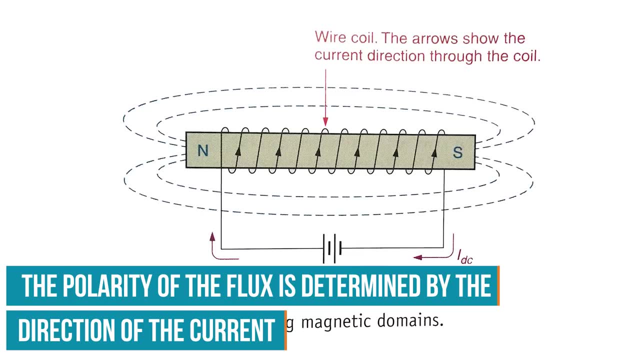 This is most effectively done by running the current through a coil of wire. When current flows through the coil, the lines of force generated by the current add together to form a bigger and stronger magnetic field. We know that if a ferromagnetic material is placed in, 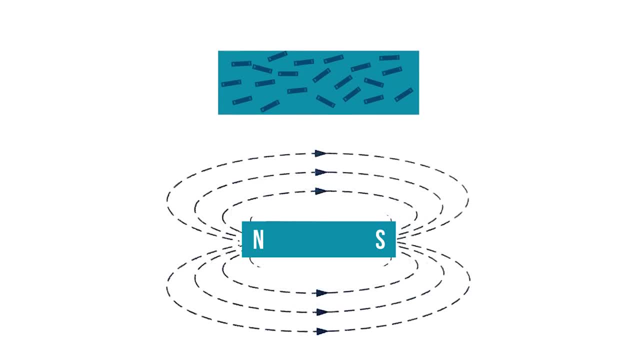 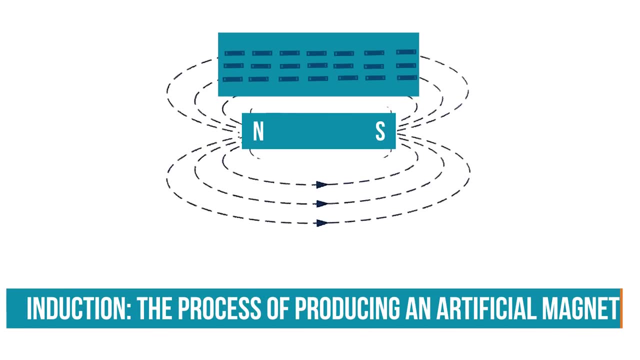 a magnetic field, its atoms will align and it will become temporarily magnetized. If an iron bar is used for the core, the lines of flux are concentrated in the bar and it becomes magnetic through induction. The coil-wrapped iron bar now acts as an electromagnet As long 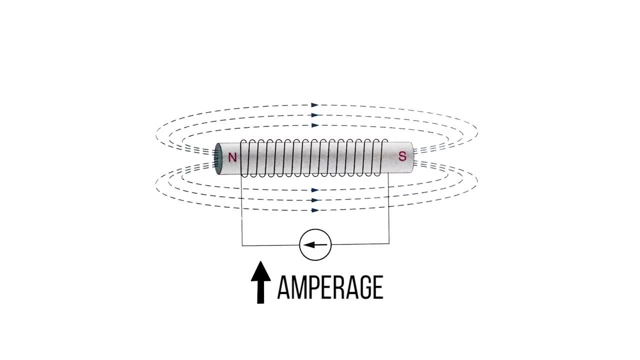 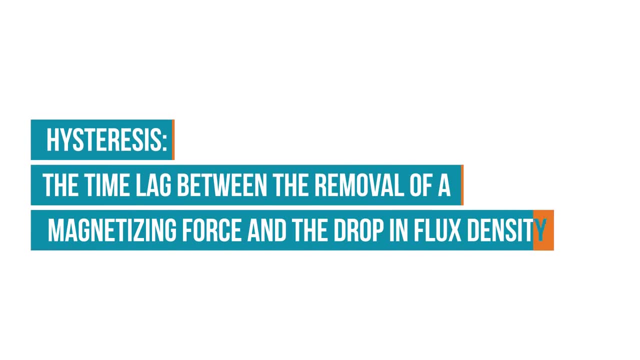 as current flows through the coil around the bar, it stays magnetized. But once current stops flowing, the bar will lose its magnetization. The time lag between the removal of a magnetizing force and the drop in flux density is known as hysteresis. The strength of an electromagnet. 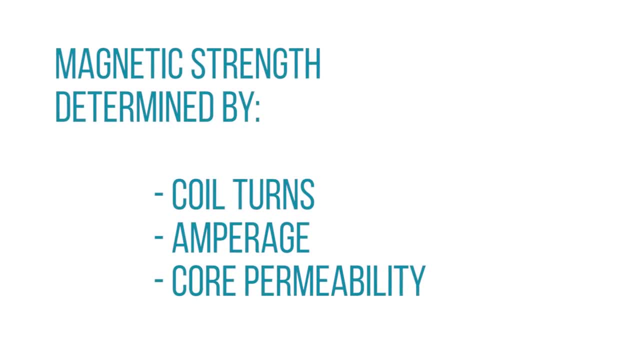 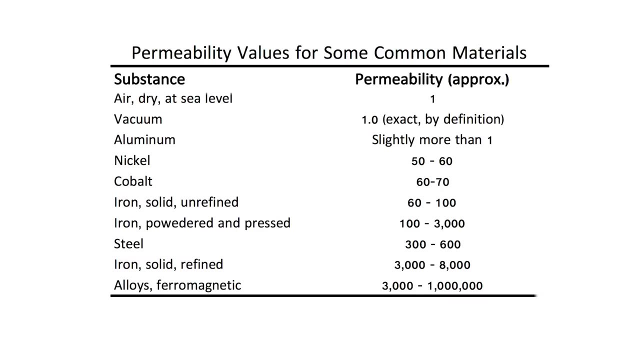 depends on three factors: the number of turns in the coil, the amperage of the current and the permeability or reluctance of the core. The core of a coil can be empty, but for electromagnets, a ferromagnetic material is often used instead due to its high permeability. The 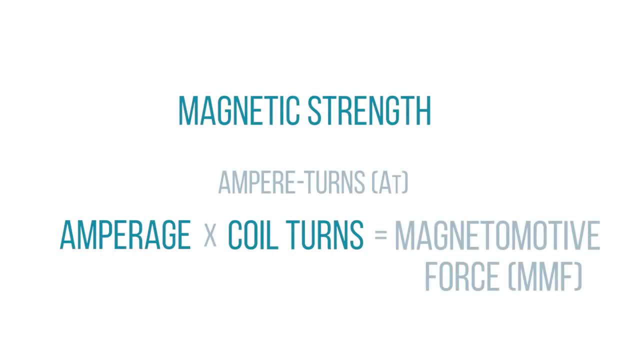 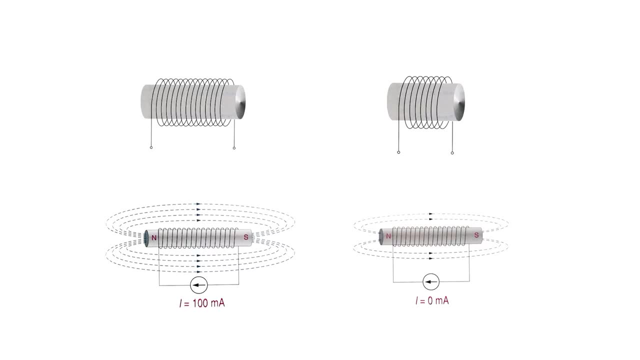 remaining two factors are combined to calculate the ampere turns or the magnetomotive force. Since magnetomotive force or MMF is calculated by multiplying the amps by the number of turns, then we know that having a higher amperage or more turns would give us a stronger magnetic.